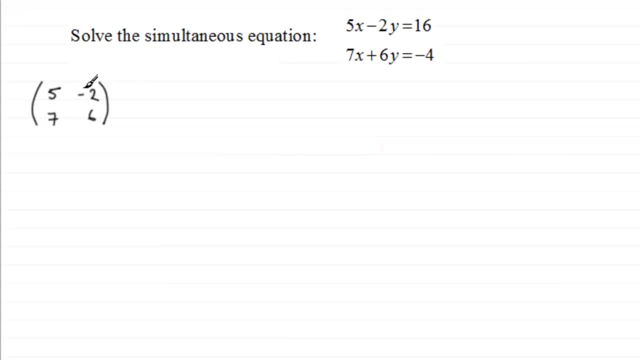 so just put seven and six there, And then we multiply this matrix by x and y, And if you do in the usual way, rows by columns, can you see that this generates five x minus two y. Look, five times x. and then we would do minus two times y, And for the 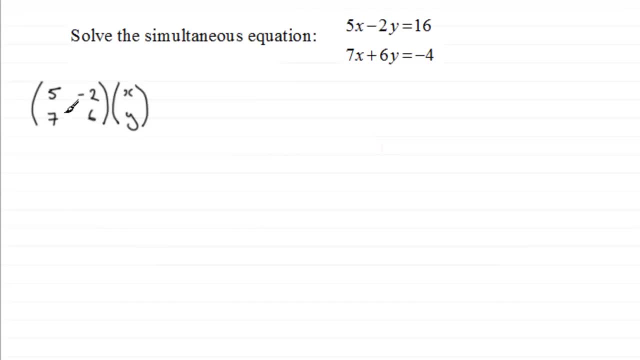 bottom row times this column. here we'd have seven times x plus six times y, generating this part of the second equation. Equate this, then, to these values here, because we would have five x minus two y would equal sixteen. And then, when it came to the bottom row, times this column: seven x plus six y. we 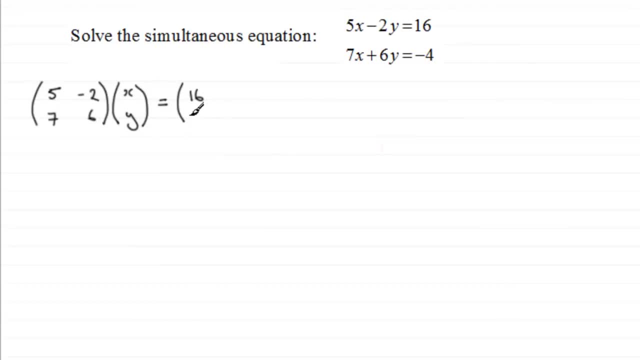 know what it gives us. it gives us minus four. So this is the matrix representation, then, of this simultaneous equation. It's just a case, now, of how we go about working out what x, y are. So let's just step to the side for a moment and just think about how we can do. 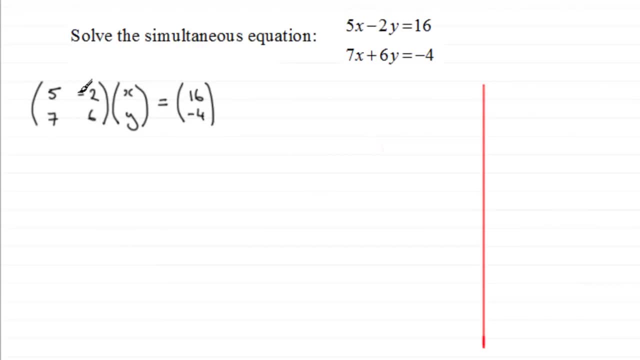 ones like this. We're always going to have a matrix here. Let's suppose that matrix is called a and we're going to multiply a with the matrix x, y, and it's going to always be equal to these two values. here Let's just say: well, in this example anyway, it's sixteen and minus four, So we'll put those in there: 16 fights. 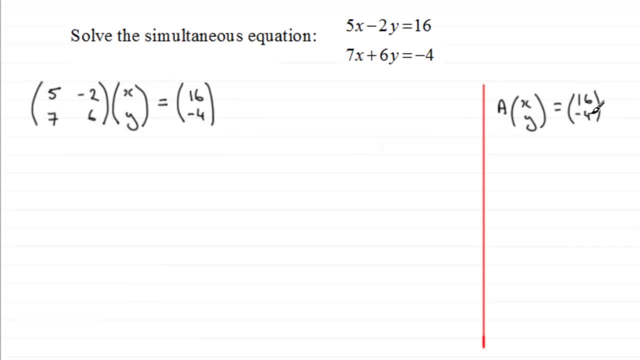 and minus four, a and b, if you like, in general. Now to solve this equation here, to get x, y, what we need to do is multiply both sides on the left by the inverse of the matrix A, In other words, a minus one there. 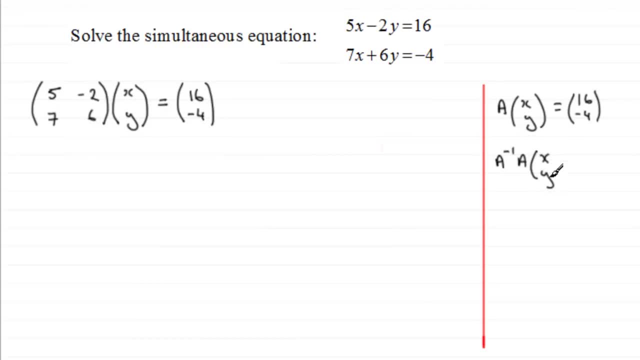 multiplied by a multiplied by x times y would give us the inverse of a multiplied by 16 minus 4.. And we should know that the inverse of matrix times a is the identity matrix. i I'll just write it in anyway. We'd therefore have: i multiplied by xy equals the inverse of a multiplied by in this: 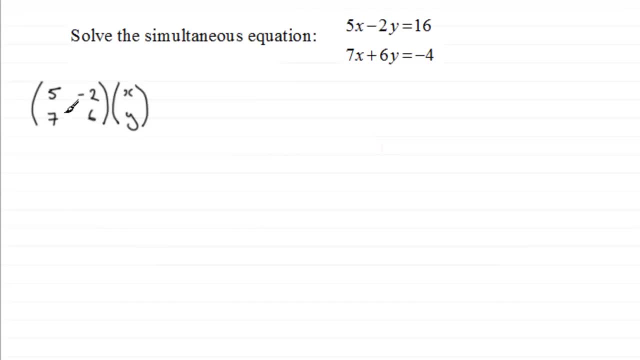 bottom row times this column. here we'd have seven times x plus six times y, generating this part of the second equation. Equate this, then, to these values here, because we would have five x minus two y would equal sixteen. And then, when it came to the bottom row, times this column: seven x plus six y. we 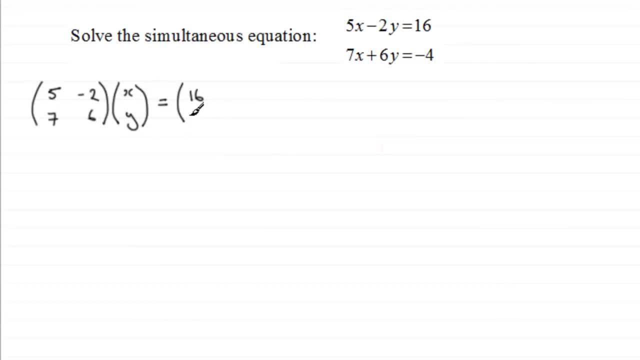 know what it gives us. It gives us minus four. So this is the matrix representation, then, of this simultaneous equation. It's just a case, now, of how we go about working out what x, y are. So let's just step to the side for a moment and just think about. 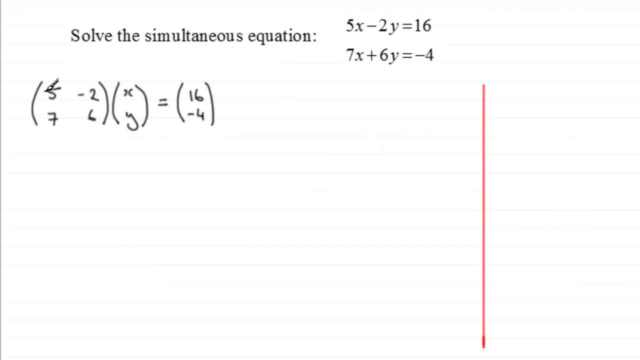 how we can do ones like this. We're always going to have a matrix here. Let's suppose that matrix is called A And we're going to multiply A with the matrix x, y, And it's going to always be equal to these two. 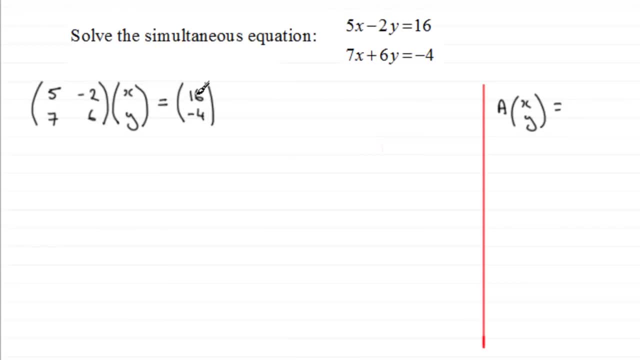 values here. Let's just say: well, in this example, anyway, it's 16 and minus 4.. So we'll put those in there, sixteen and minus four, a and b, if you like, in general. Now to solve this equation here, to get XY, what we need to do is multiply both sides. 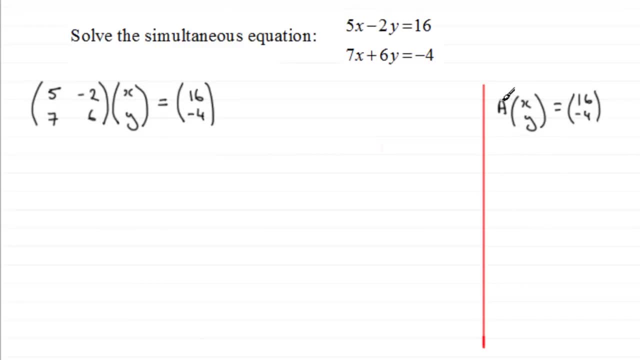 on the left, by the inverse of the Matrix A, In other words A minus one there. Multiplies them together, See multiplied by a multiplied by x times y would give us the inverse of a multiplied by 16 minus 4.. And we should know that the inverse of matrix times a is the identity matrix i. I'll just write: 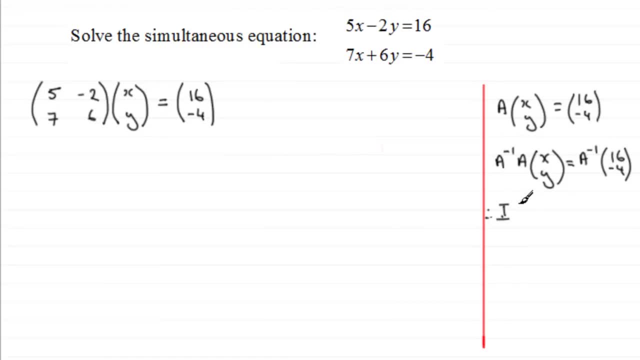 it in anyway. We'd therefore have: i multiplied by xy equals the inverse of a multiplied by, in this case, 16 minus 4, or whatever. your equation has Now the identity matrix times any matrix leaves it unchanged, The result that we should be familiar with in early videos that I've done for you. 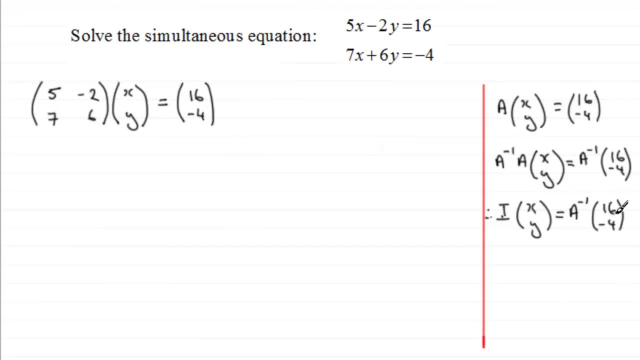 case 16 minus 4 or whatever your equation has Now the identity matrix times any matrix leaves it unchanged, The result that we should be familiar with in early videos that I've done for you. So we're just left with xy. xy equals the inverse of a, then multiplied by 16 minus 4, and this is the result that we always 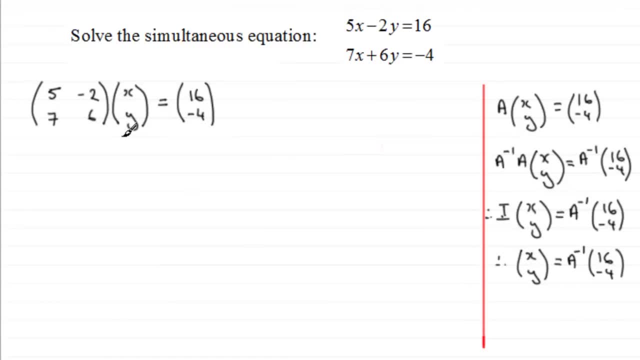 are going to use. If we want to find xy, all we need to do is multiply 16 minus 4- whatever values we've got here- by the inverse of this matrix, and this matrix must be on the left of these values. Okay, Like we've got here, so, assuming that I'm familiar with this, that if I was answering this question. 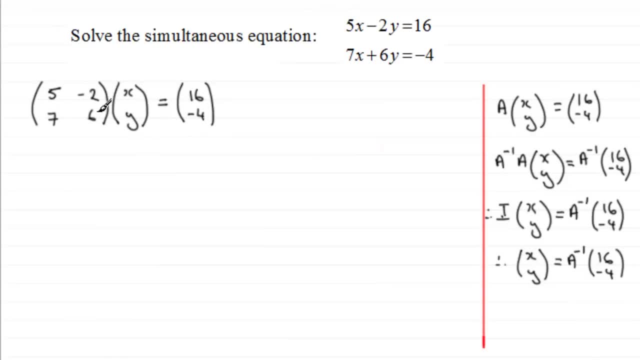 I would want to work out first of all what the inverse of this matrix is. So I'm going to call it a. So I'd say, let a be that matrix a equal the matrix 5 minus 2, 7, 6.. Now I'm assuming that 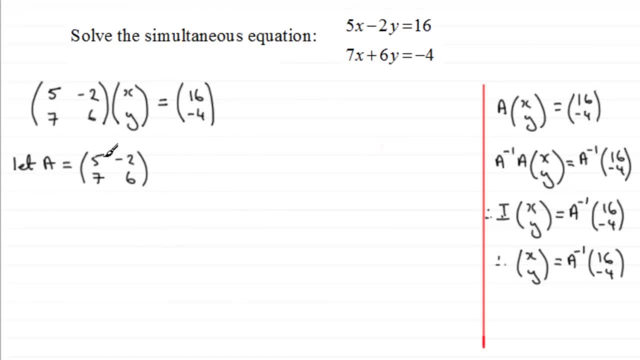 you're familiar with finding inverses of matrices, Two by two matrices. If not, just go on my website and look in this series under inverse matrices and you'll find an explanation there. But we had to find out the determinant of the matrix A. Remember, the determinant of the matrix A was to multiply 5 and 6 together and then. 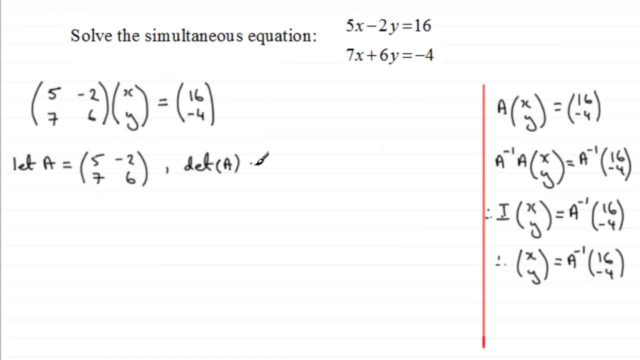 subtract 7 and times minus 2.. So if we do that, we get 5 times, which is 30. then subtract 7 times minus 2, subtract then minus 14. what does that give us? it gives us 44. so when it comes to working out what the inverse of a is, 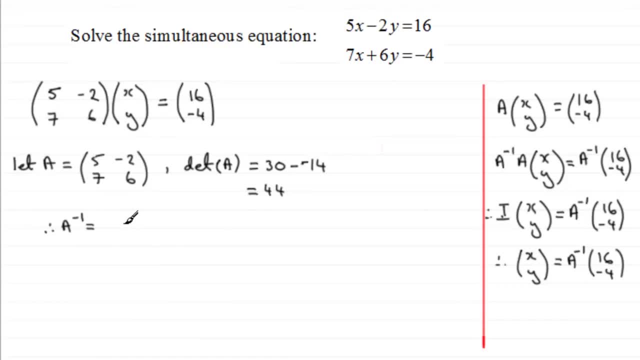 we can say: therefore, the inverse of a is equal to- and it was always equal to 1 divided by the determinant of a, so that's 1 over 44. and then what we did was we switch these two elements around. so 6 goes there, 5 goes there and we 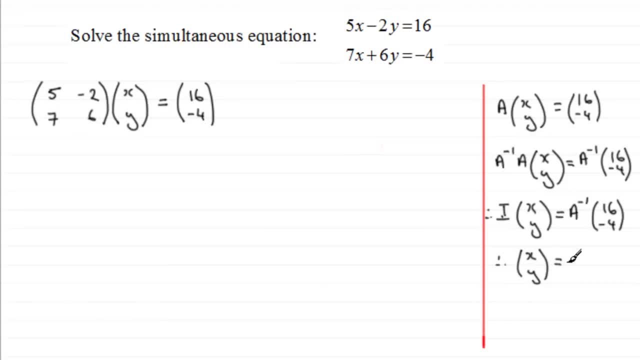 So we're just left with xy. xy equals the inverse of a, then multiplied by 16 minus 4, and this is the result that we always are going to use. If we want to find xy, all we need to do is multiply 16 minus 4, whatever values. 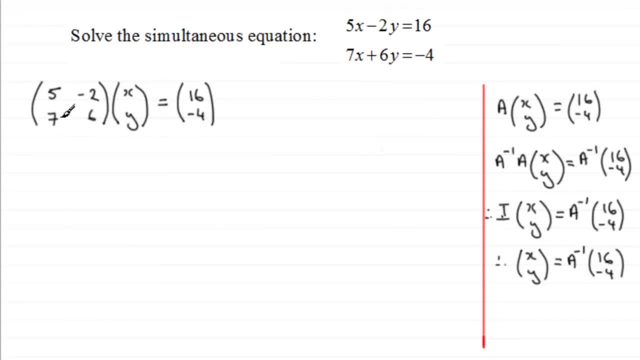 we've got here by the inverse of this matrix and this matrix must be on the left of these values. Okay, Like we've got here, so, assuming that I'm familiar with this- that if I was answering this question I would want to work out first of all what the inverse of this matrix is. So I'm going to call. 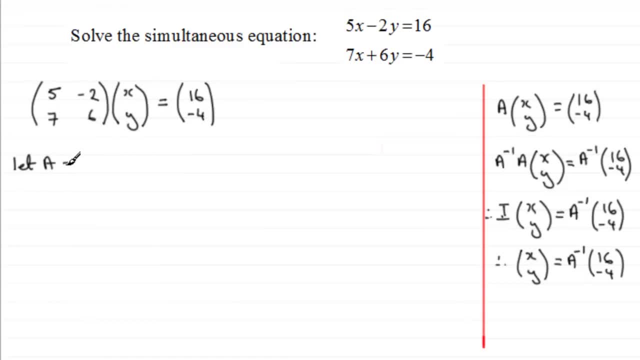 it a. So I'd say let a be that matrix a equal, the matrix 5 minus 2, 7, 6.. Now I'm assuming that you're familiar with finding inverses of matrices, Two by two matrices. If not, just go on my website and look in this series under inverse. 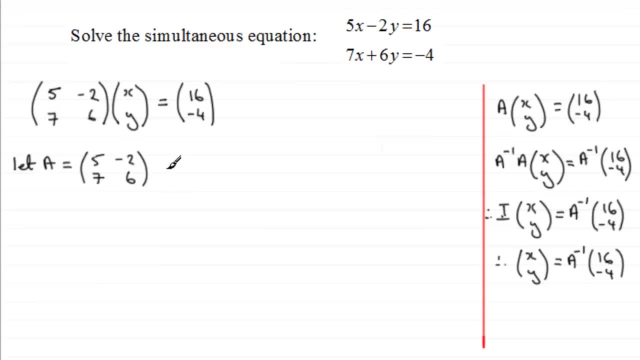 matrices and you'll find an explanation there. But we have to find out the determinant of the matrix a. Remember? the determinant of the matrix a was to multiply 5 and 6 together and then subtract 7 and times minus 2.. So if we do that, we get 5 times 6,. 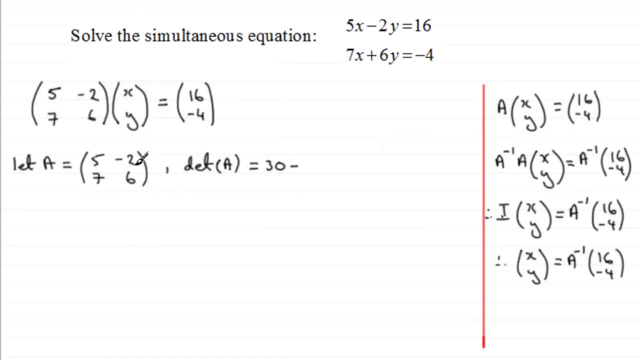 times 6, which is 30. then subtract 7 times minus 2, subtract then minus 14. what does that give us? it gives us 44. so when it comes to working out what the inverse of a is, we can say: therefore, the inverse of a is equal to, and it was. 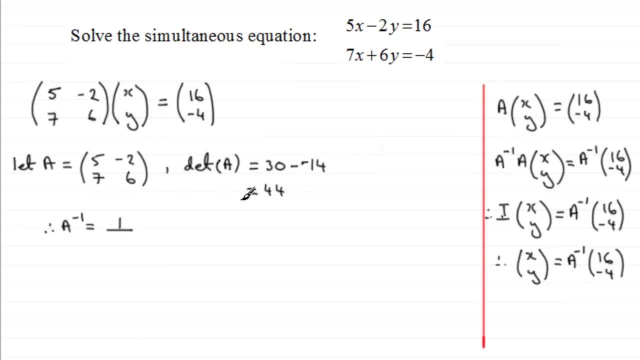 always equal to 1 divided by the determinant of a, so that's 1 over 44. and then what we did was we switch these two elements around, so 6 goes there, 5 goes there, and we change the sign of these two elements, so that's minus 7. and then 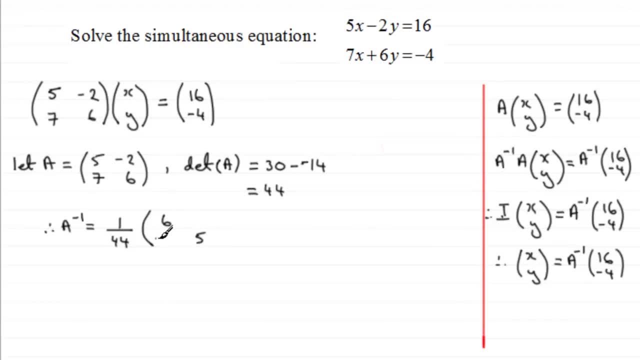 change the sign of these two elements so that's minus 7, and then changing the sign on the minus 2 just gives us the 2, so there's our inverse matrix. we could write this as 6 over 44, 2 over 44, minus 7 over 44 and 5 over 44. it's up to you. 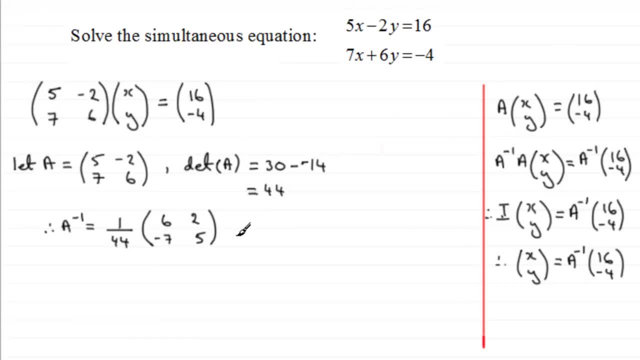 but I'm just going to leave it like this. I find it easier for problems like this. so, by this idea, then, it means that therefore, XY- okay- is going to equal the inverse of a. let's just put it then as 1 over 44, and then 6, 2 minus 7 and 5, and we: 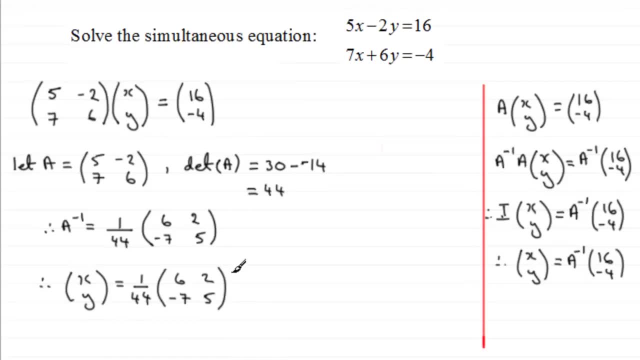 multiply this by 16 minus 4, so 16 minus 4, and so the first thing I'd want to do now is just leave the 1 over 44 there and we'll multiply 6, 2 minus 7, 5 with the 16: 4. that's going to give us a matrix. 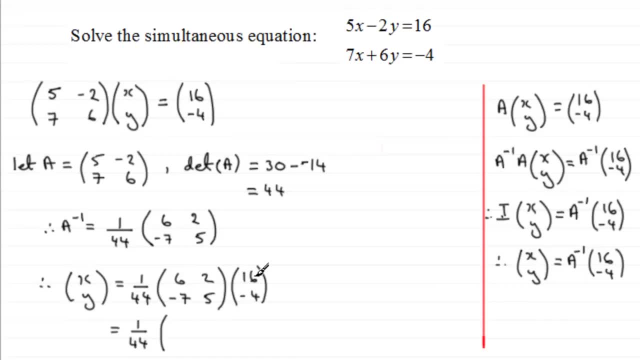 something like this: we're going to do 6 times 16, which is going to be 96, and then add it to 2 times minus 4, which is minus 8, so you've got 96 minus 8, and that gives us 88. 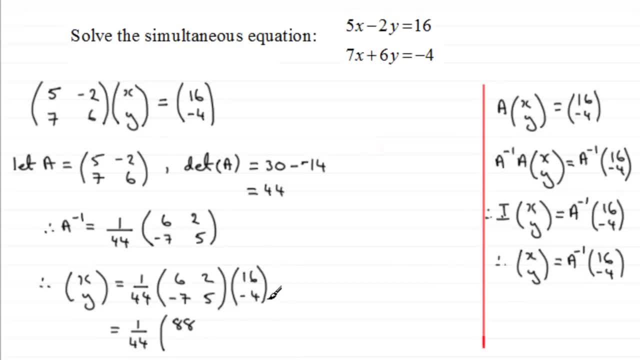 lastly, we do minus 7, 5 times 16 minus 4, so that'd be minus 7 times 16, which is minus 112, and then add that to 5 times minus 4, which is minus 20. minus 112, minus 20 is minus 132. now I can take 144th of each of these two values divide. 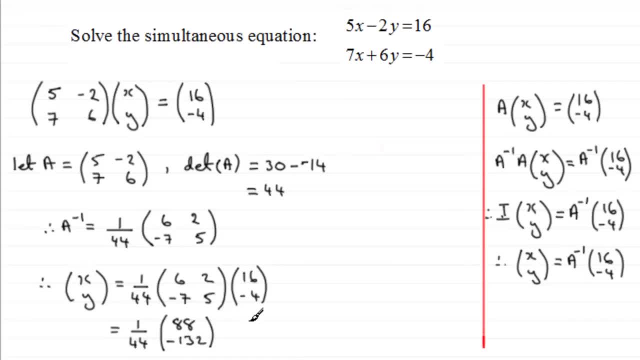 them by 44, in other words, and that means that I end up with 2: 88 divided by 44 is 2, and then minus 132 divided by 44 is minus 3. so you can see that XY equals 2 minus 3. so at the end of the day, what we have is: 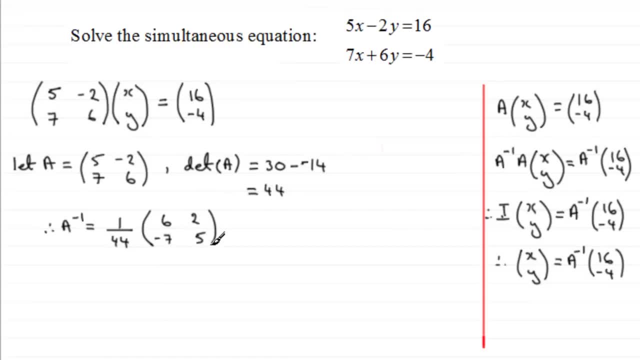 changing the sign on the minus 2 just gives us the 2, so there's our inverse matrix. we could write this as 6 over 44, 2 over 44, minus 7 over 44 and 5 over 44. it's up to you, but I'm just going to leave it like this. 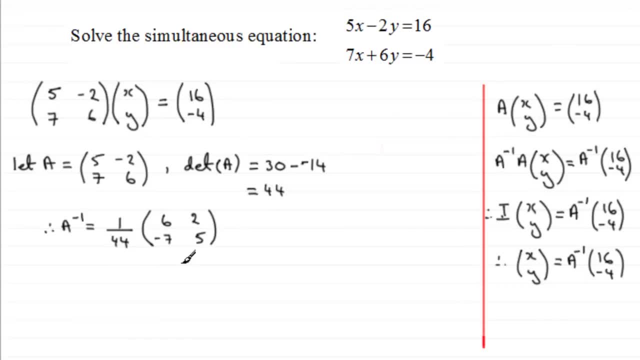 I've find it easier for problems like this. so by this idea, then, it means that therefore, XY- okay- is going to equal the inverse of a. let's just put it then as 1 over 44, and then 6, 2 minus 7 and 5, and we multiply this by 16 minus 4, so 16. 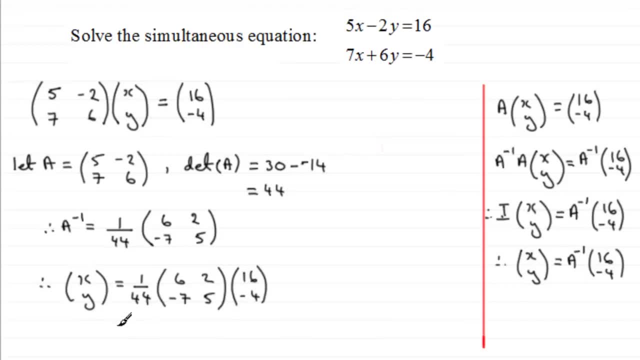 minus 4, and then we multiply this by 16 minus 4, and then we multiply this by 16 minus 4, and so the first thing I'd want to do now is just leave the 1 over 44 minus 4, and so the first thing I'd want to do now is just leave the 1 over 44. 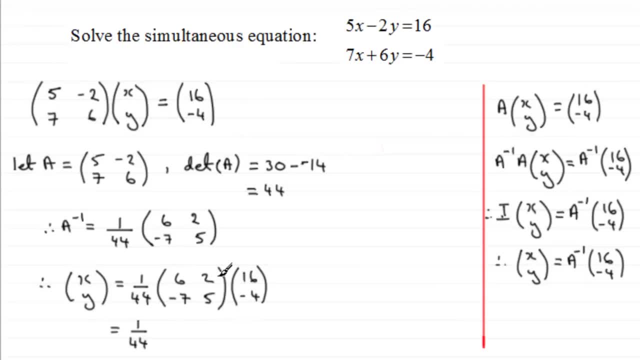 there and we'll multiply 6, 2 minus 7, 5 with the 16, 4. that's going to give us a matrix, something like this: we're going to do 6 times 16, which is going to be 96, and then add it to 2 times minus 4, which is minus 8. so you've got 96 minus 8, and 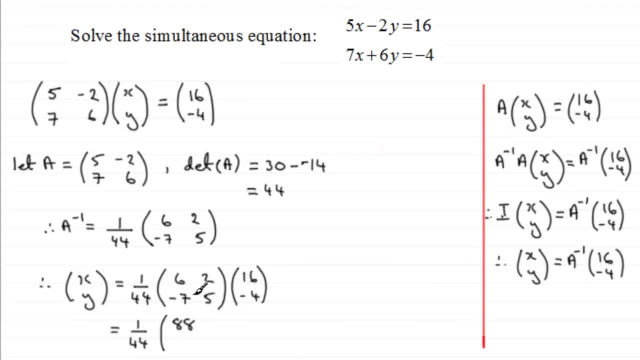 that gives us 88. lastly, we do minus 7, 5 times 16 minus 4. so be minus 7 times 16, which is 112, and then add that to 5 times minus 4, which is minus 20 minus 112. minus 20 is: 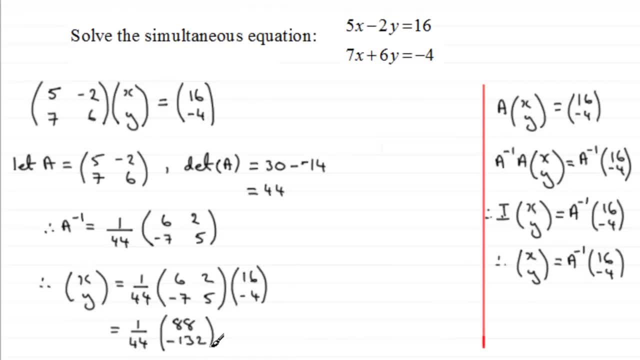 minus 132. now I can take 144th of each of these two values, divide them by 44 in these two values, divide them by 44, in other words, and that means that I end up with 2: 88 divided by 44 is 2, and then minus 132 divided.